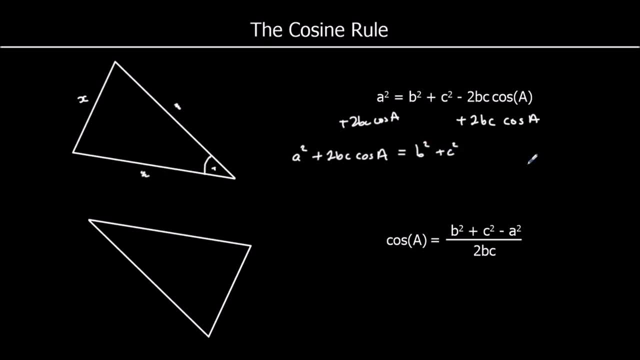 plus c squared. Then I subtract a squared from both sides, So take a squared away from both sides, Which just leaves me with 2bc cos a on one side. So I take a squared from both sides And I've got b squared plus c squared, minus a squared on the other. 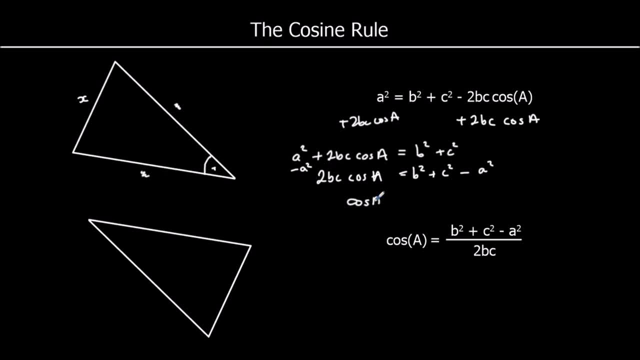 I then divide both sides by 2bc And we get cos a equals b squared plus c squared minus a squared over 2bc. So this is the formula for working at an angle, And we can find an angle in a triangle when we know all three of the sides. 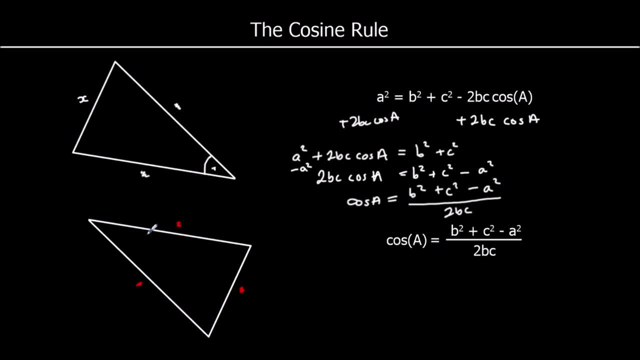 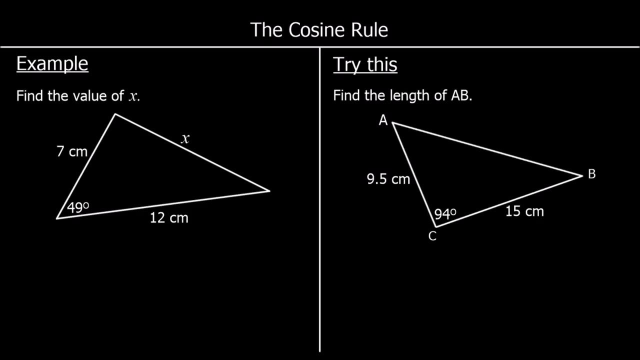 So when we know all three sides of a triangle, we can work out any of the angles using the cosine rule. So let's have a look how this works. The first question: find the value of x. So we've got two lengths and the angle in between them. 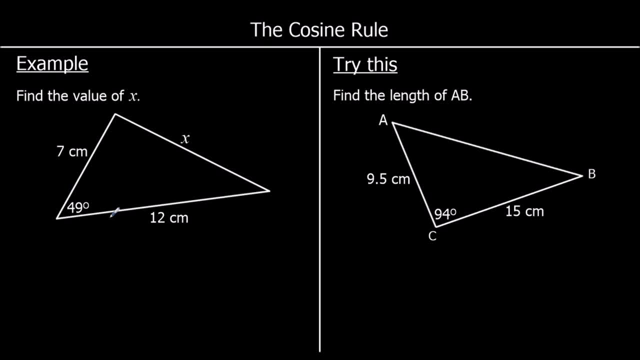 So two lengths and the angle in between them. That's what we're looking for with the cosine rule And we're finding The length. So we're going to use the rule: a squared equals b squared plus c. squared minus 2bc cos a. 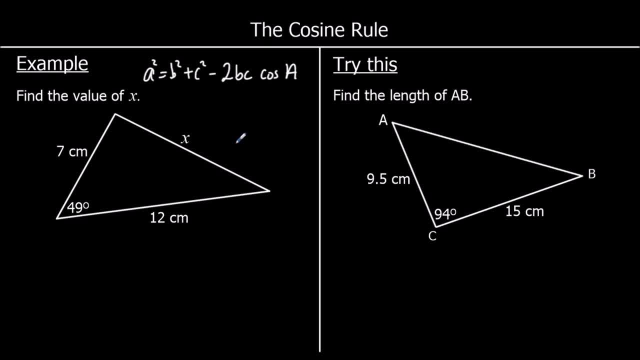 So let's label it. The big A is the angle, So there's only one angle. we know That's big A And that's opposite little a, which is what we're working out. The other two are called b and c. 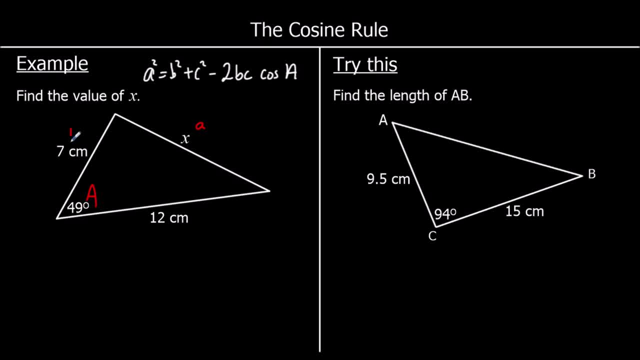 And it doesn't matter which way round we put them. So we just put b And c So we can substitute our values into our formula now. So we've got x squared Equals 7 squared Plus 12 squared, Minus 2 times 7 times 12, cos 49.. 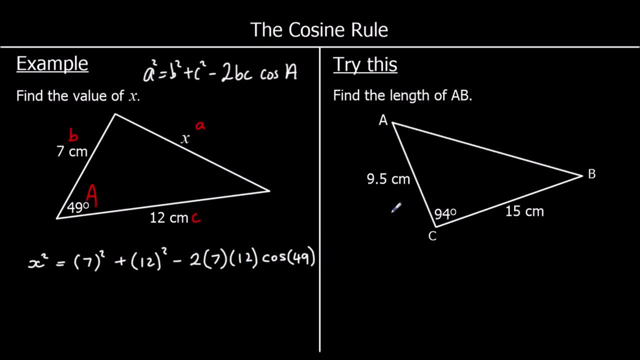 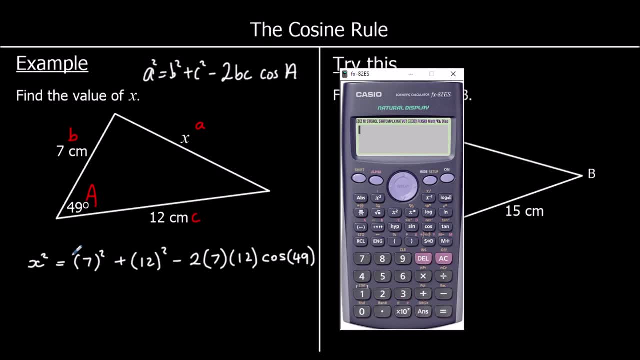 Cos 49. So we've substituted our values in. Now we can pick up our calculator and we can actually type this whole side in. So 7 squared plus 12 squared minus 2 times 7 times 12, cos 49.. So I'm going to type that whole thing in. 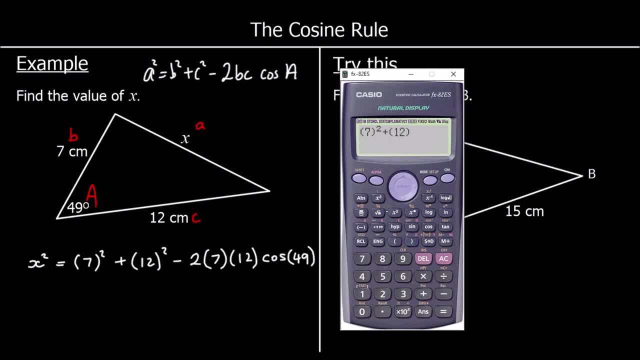 I use brackets when I substitute numbers into the calculator. It's a good habit to be in, Because when you have negative numbers your calculator doesn't make a mistake. So I've typed that whole side in to the calculator And I've got 82.78 and so on. 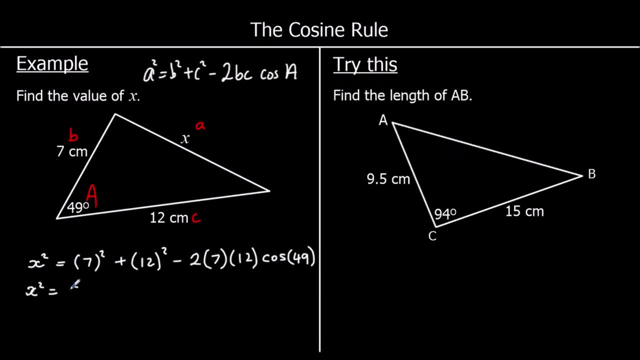 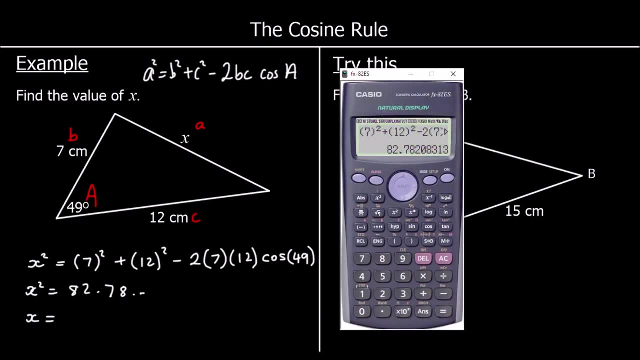 So x squared is equal to 82.78, and so on. I need to find x, not x squared, So I need to square root. So square root my answer And I'll give my answer to two decimal places. So that's going to be 9.10.. 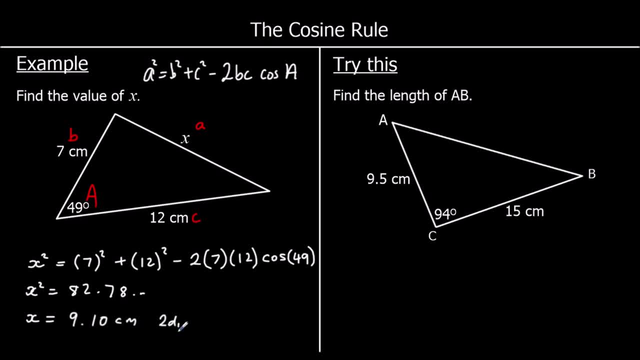 And it's centimetres to two decimal places. Okay, a question for you to try. So pause the video And give it a go. Okay, so we've got two lengths and the angle in between them. We are finding the other length. 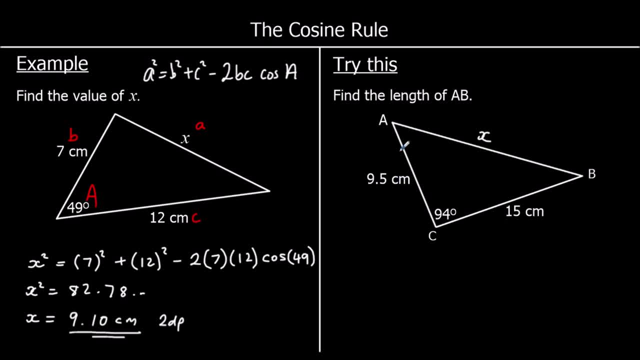 So we're going to use the cosine rule, And it's for lengths. So we're going to use: a squared equals b squared plus c squared minus 2bc, cos a, Okay, And to label it, The angle is big A. What we're working out, opposite, it is little a. 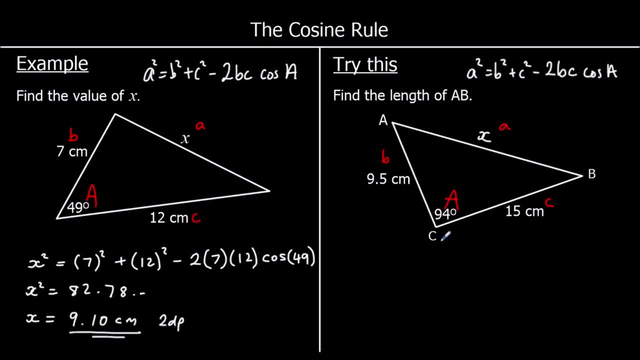 And the other two are b and c. either way around, It doesn't matter which way you put them, And we'll grab the calculator. No, we won't, We'll substitute in first. So we're going to have x squared equals 9.5 squared plus 15 squared. minus 2bc cos a. So we're going to have x squared equals 9.5 squared, plus 15 squared minus 2bc cos a. So we're going to have x squared equals 9.5 squared plus 15 squared minus 2bc cos a. 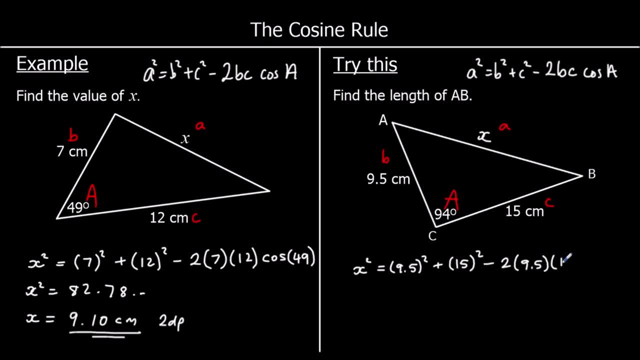 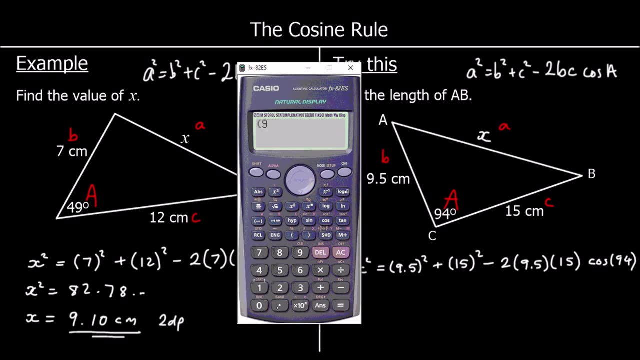 Times 2 times 9.5 times 15, cos 94.. So we're going to type the whole of the right side in. So we've got 9.5 squared plus 15, squared minus 2 times 9.5 times 15.. 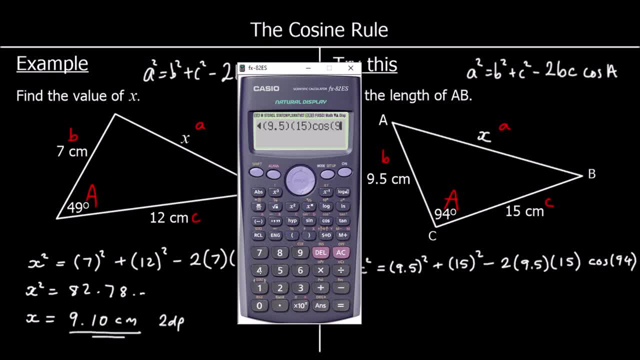 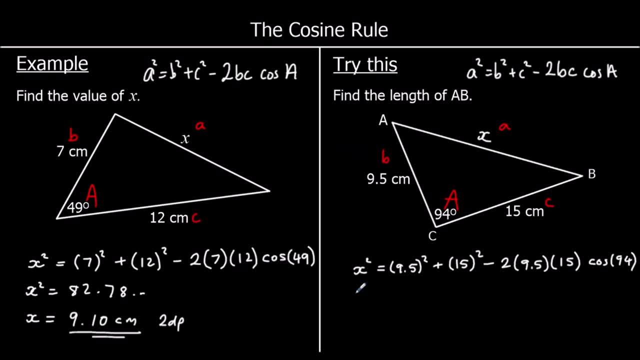 So we've got 9.5 squared plus 15 squared minus 2 times 9.5, times 15 squared minus 2.. 15 cos 94.. So we've got 335.13 and so on. So 335.13, dot, dot, dot. 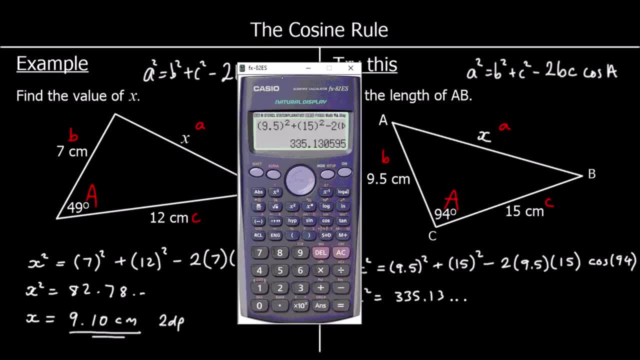 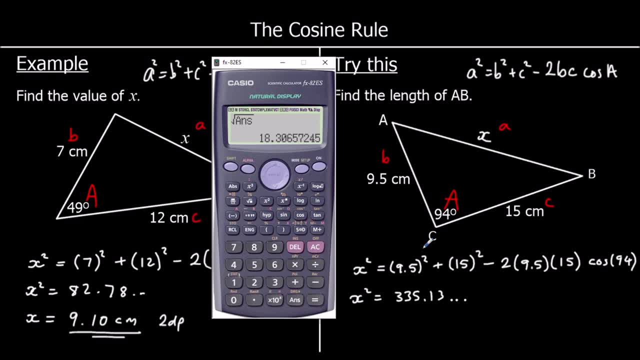 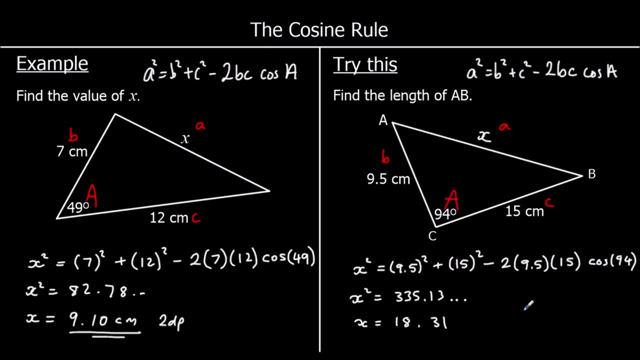 That's x squared. To get x we need to square root. So I'm going to press square root. answer And that's 18.31 to two decimal places. So x equals 18.31.. It's in centimetres and it's to two decimal places. 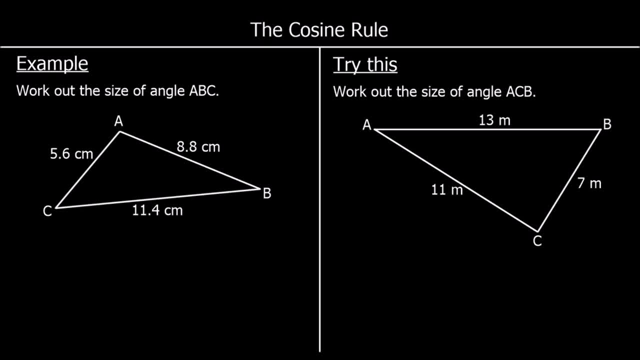 Okay, Work out the size of angle ABC. So this time we're working on angle Angle. ABC is this angle here, A to B to C? So that's our x, The cosine rule. We can use the cosine rule when we know all three lengths and we want to work out an angle. 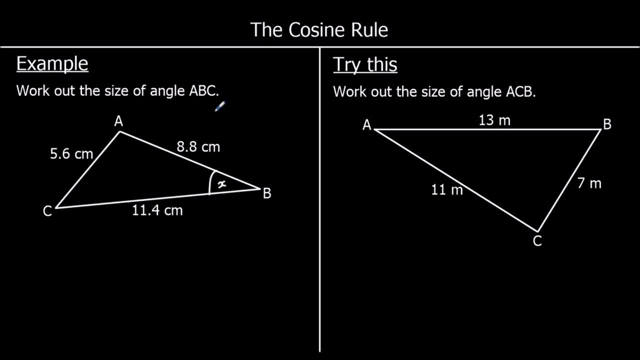 So it is the cosine rule And we are going to use cos A equals B squared plus C squared minus A squared over 2BC. So it's labelled the triangle. Big A is our angle. That's what we're working out. Opposite big A is little a and the other two are called B and C. 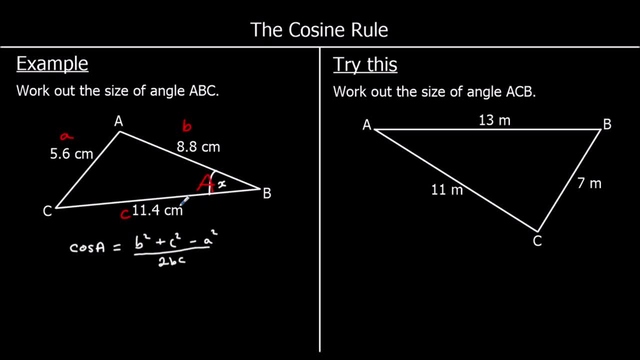 It doesn't matter which way around we put B and C. I could have put them the other way around, It wouldn't make a difference to the answer. So let's substitute in: So we've got cos x this time, And that's B squared, which is 8.8 squared. 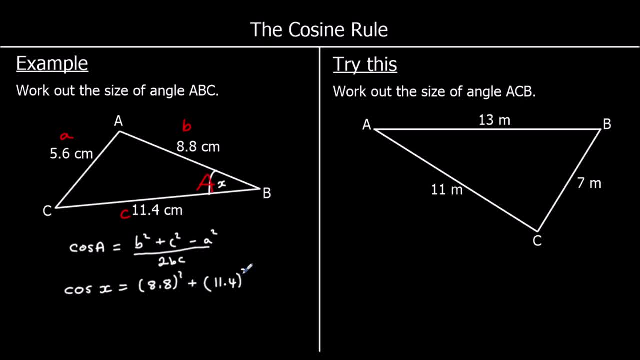 Plus C squared, 11.4 squared Minus A squared, which is 5.6 squared Over 2BC, So 2 times 8.8 times 11.4.. So we're going to type this side into the calculator. 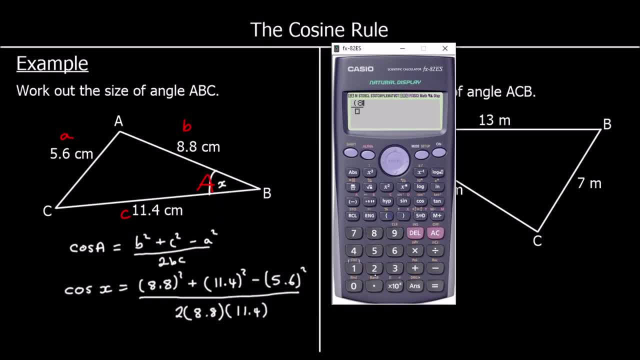 So fraction button: 8.8 squared plus 11.4. squared Minus 5.6, squared over 2 times 8.8 times 11.4.. So that's come out as 0.877, and so on. 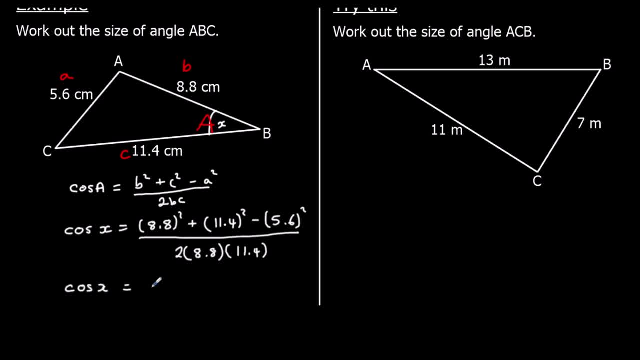 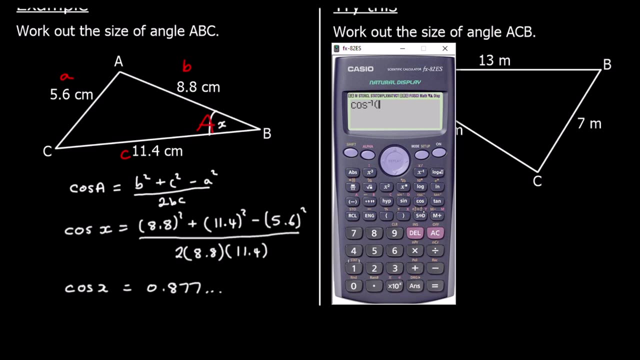 So cos x equals 0.877, and so on. How do we get cos away from x? How do we get x by itself? What's the opposite of cos? We need to shift cos. So shift cos, our answer. And we've got 28.67.. 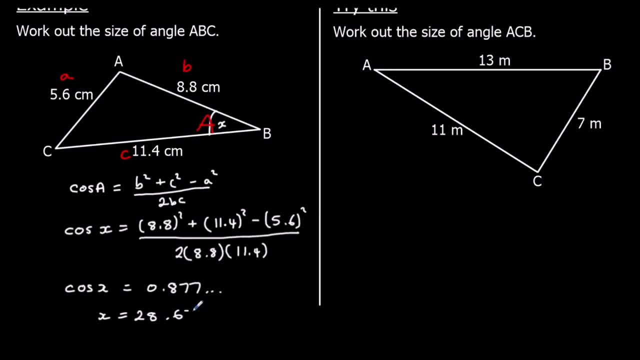 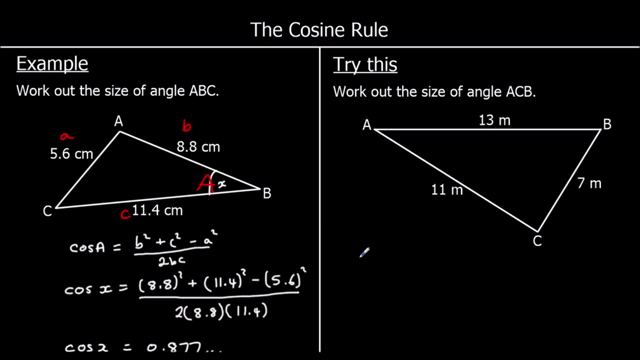 x is 28.67 degrees to two decimal places again, And one for you, And one for you to try. So pause the video, Give it a go And press play when you're ready for the answer. Okay, Angle ACB. 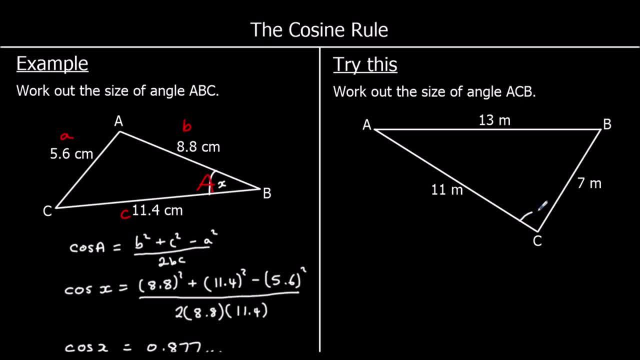 A to C to B. That's what we're working out And we're using the cosine rule. We can use the cosine rule because we know all three lengths And we are working out one of the angles. So it's going to be: cos A equals b squared plus c squared minus a squared over 2bc. 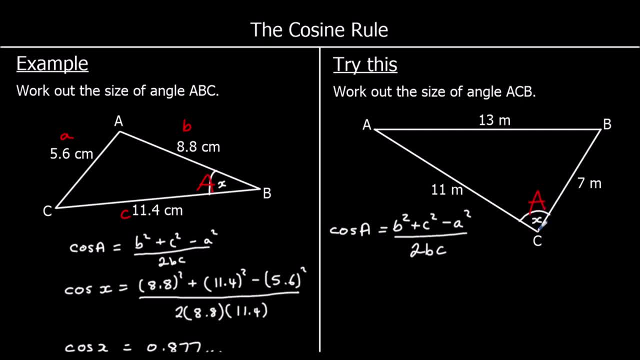 Big A is going to be our angle that we're working out. Opposite big A is little a And the other two are b and c And it doesn't matter which way around you put b and c, So substituting in, we're going to have cos x. 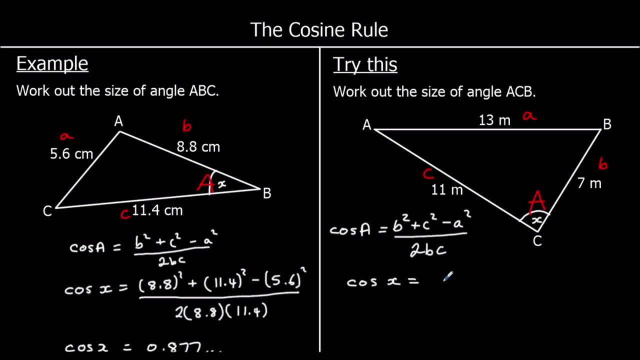 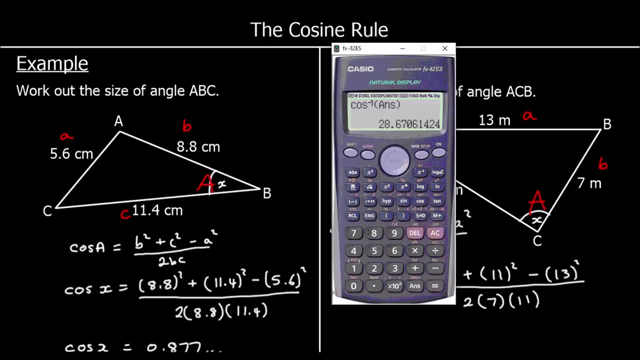 cos x is equal to b squared, which I've got a, 7 squared plus c squared, so 11 squared minus a squared, which is 13 squared over 2 times b times c. I'm going to type this into the calculator. 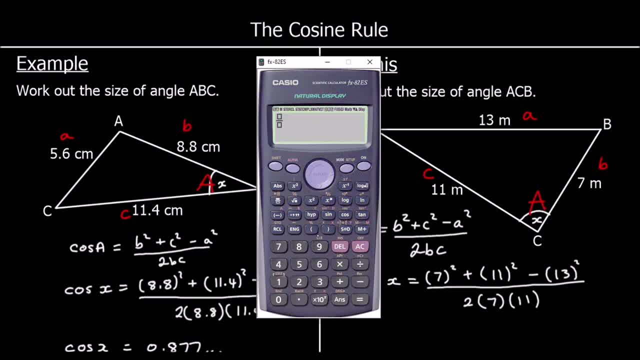 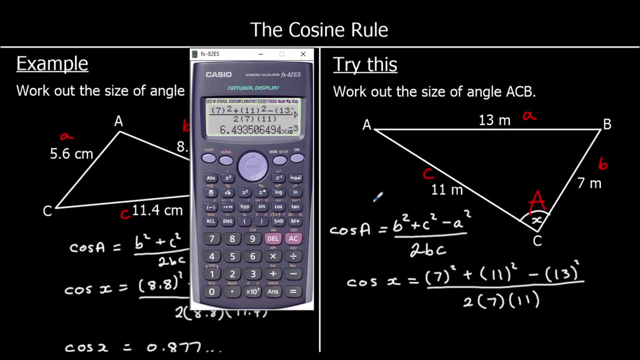 It's a fraction button. I've got 7 squared Plus 11 squared minus 13, squared over 2 times 7 times 11.. So I've got 1 over 154, or, as a decimal, a really tiny number. 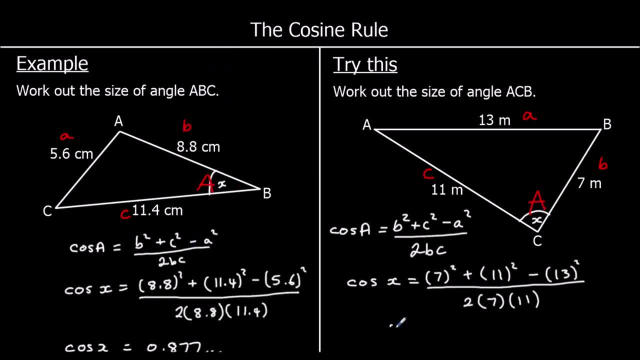 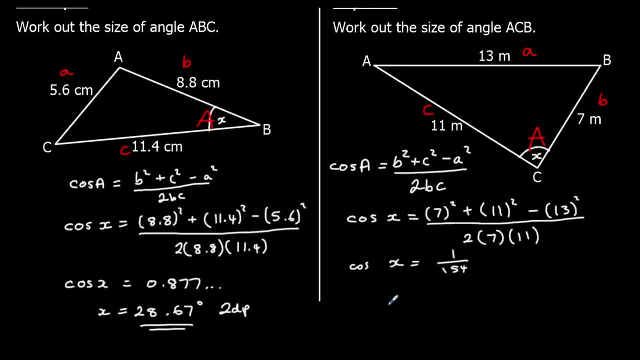 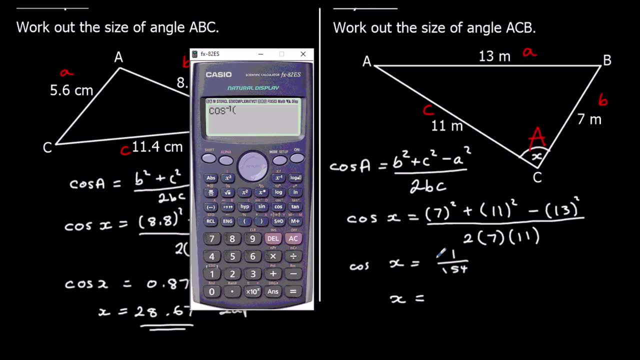 I'll put 1 over 154.. So cos x equals 1 over 154.. We need to get x by itself, so we shift cos, Get cos away from x, shift cos the answer, And that has given us 89.63.. 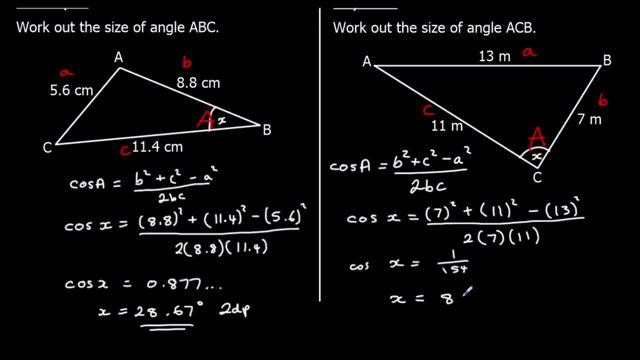 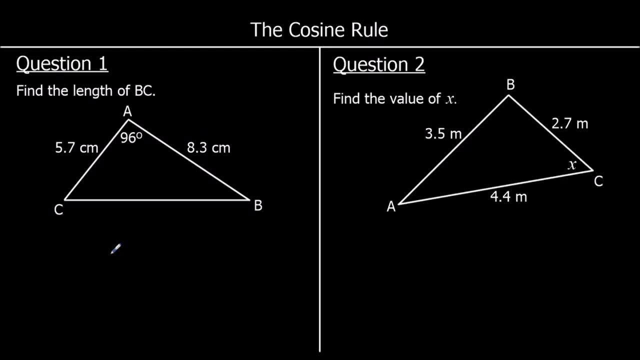 So 89.63 degrees to two decimal places. So that's that And that is the answer for the question. That's the answer for the question. That's the answer for the question. That's the answer for the question, And there are two questions here. 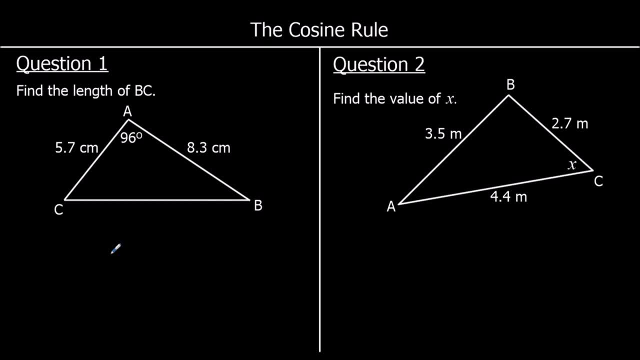 So pause the video, have a go at these questions to finish up, and then I'll go through the answers after. Okay, question one: Find the length of bc. So we're finding this length. We know two lengths and the angle between them. 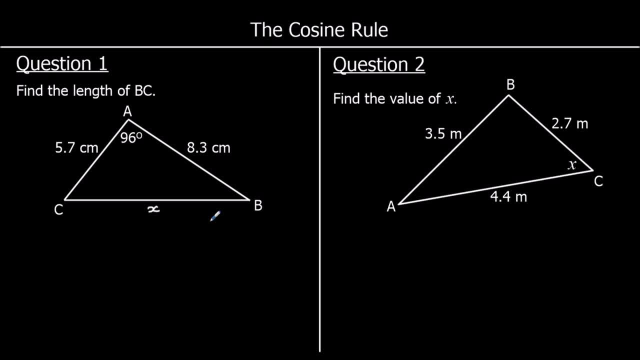 so we can use that to find the length of bc. So we can use that to find the length of bc. use the cosine rule. and the cosine rule says to find the length we want: a squared equals b. squared plus c. squared minus 2, BC cos a, we're going to have big. 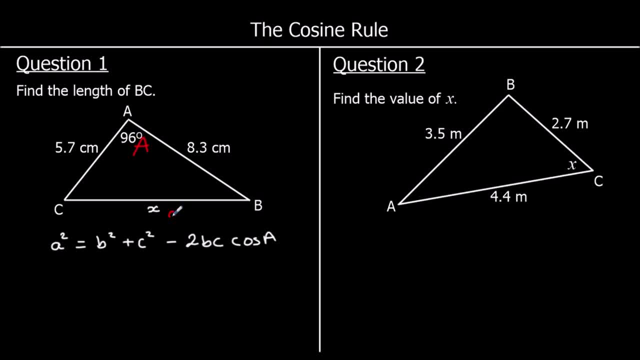 a as our angle opposite, it will be little a, which is what we're working out, and the other two, in either way round, are called B and C. so substituting in, we've got x squared equals five point seven squared plus eight point three squared minus two times five point seven times eight point three, cos 96, and I'm 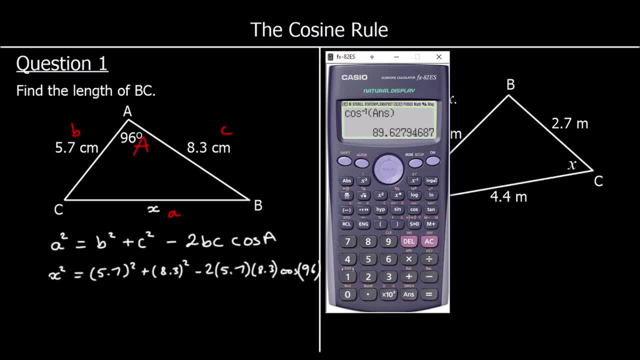 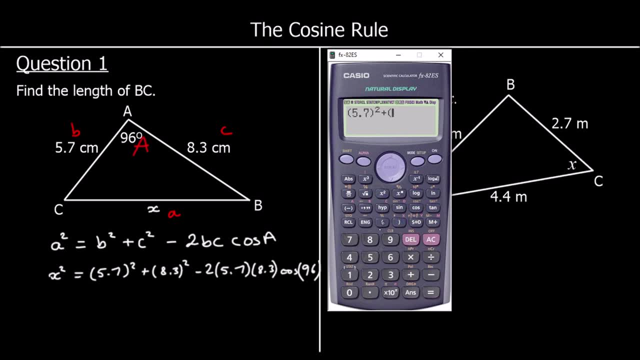 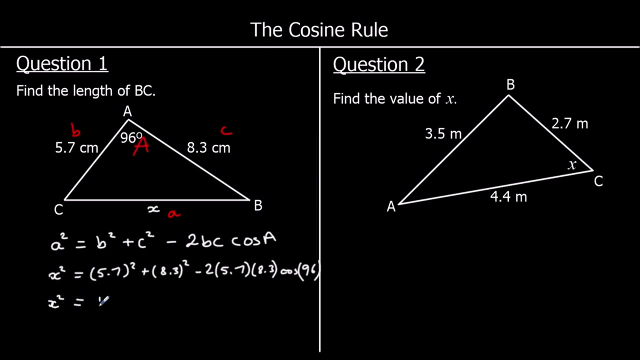 gonna. I'm gonna type this all into the calculator. So 5.7 squared plus 8.3 squared minus 2 times 5.7 times 8.3, cos 96.. So I've got 111.27.. So x squared is 111.27.. I need to get x by itself. 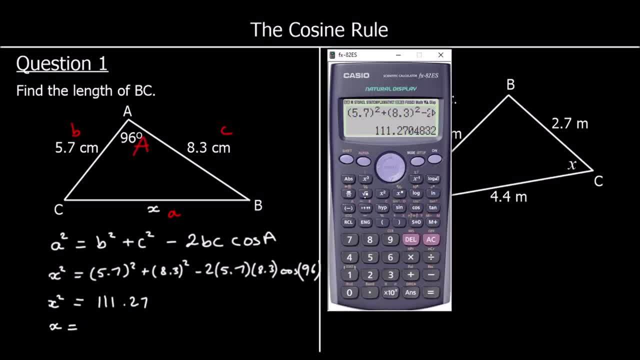 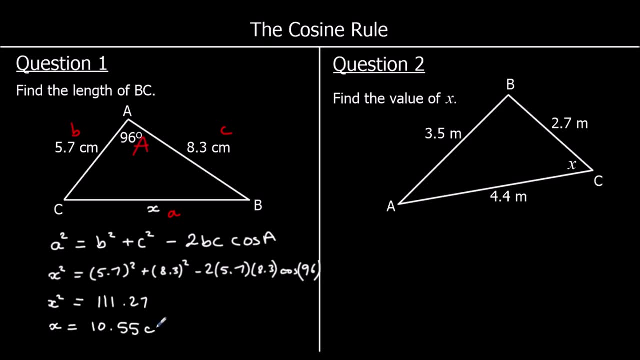 So I'm going to square root. Square root my answer, which, to two decimal places, is 10.55.. So x is 10.55.. It's in centimetres to 2dp. And question two: find the value of x. So we're finding an angle and we know all three. 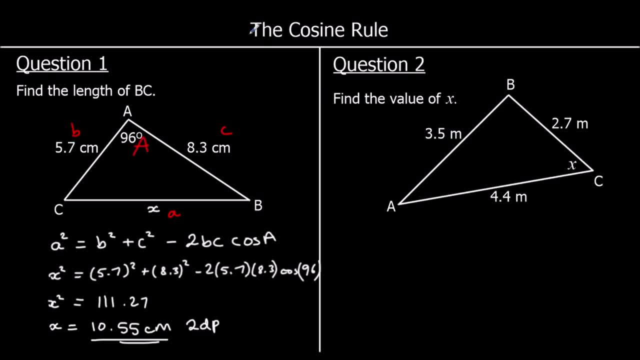 lengths. So we can use the cosine rule. I'm going to use the rearranged version, which is cos a is b squared plus c squared minus a squared over 2bc, And we're going to have big A as x, the angle little a opposite. 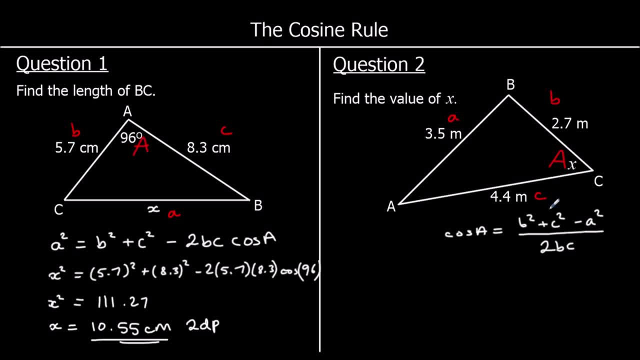 it and b and c either way around as the other two. So let's substitute in: So we've got a. So substituting in, we have: cos x equals 2.5 squared plus 2.3 squared plus 2.7 squared.